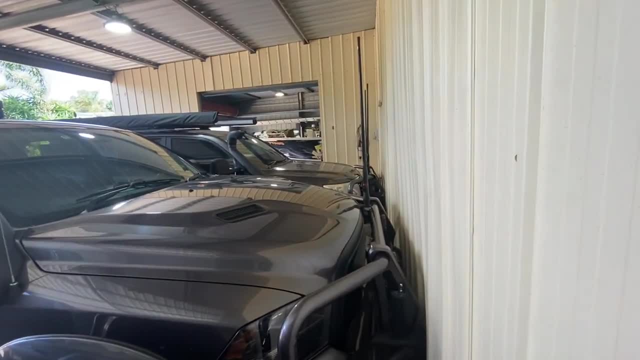 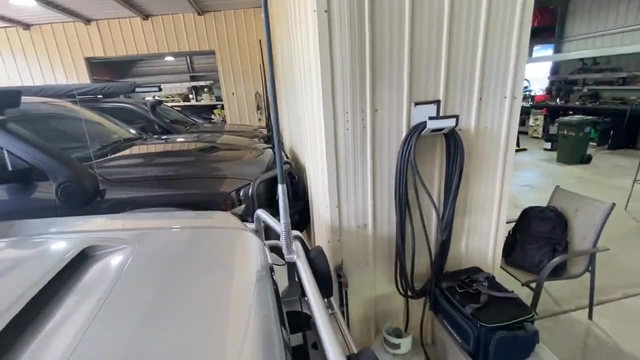 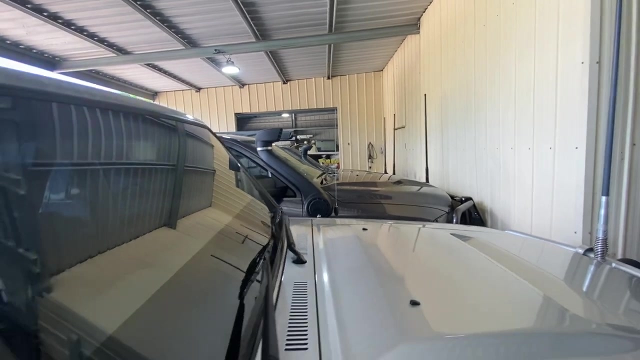 And matey's got a two inch lift kit in the 200, which has probably dropped a bit because of the age on it. It's a bit hard with the video, But have a look at that all together. going through to the windscreens, not much difference in the car's line of the windscreens up. 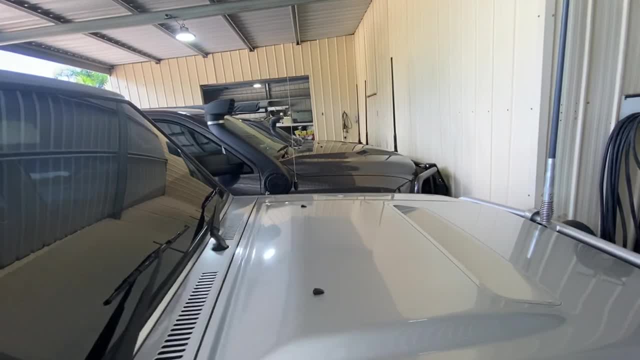 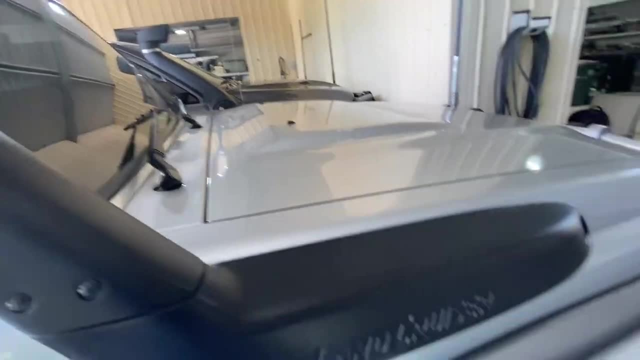 If you look along them all, pretty much neither here nor there in the same length from the Bulba to the windscreens smidgen higher in the ram. Not sure where the wheelbases are. can't see that. Keep going through. 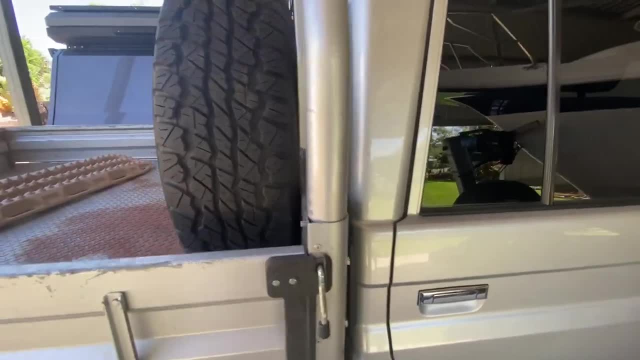 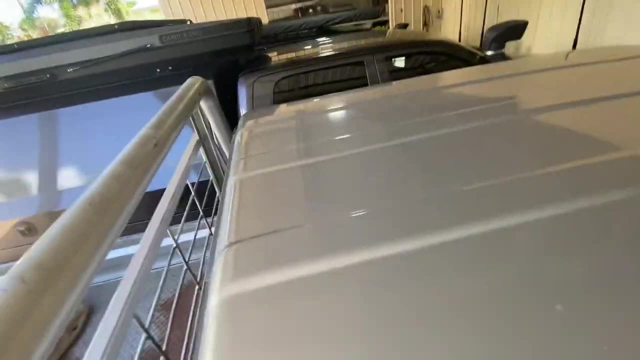 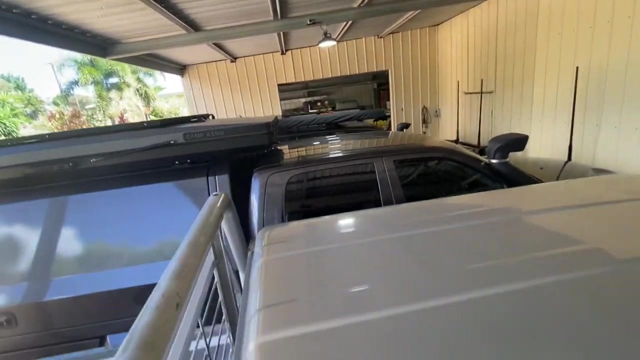 Now look at the back door. From the front door to the back door it actually would you believe there's not much difference in where the door's finished And the length 200, if you can see over there. so they're the same. 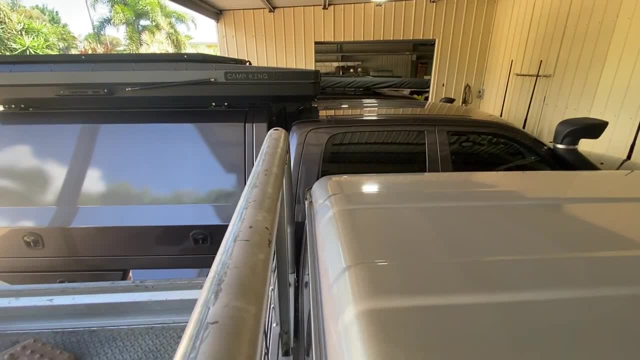 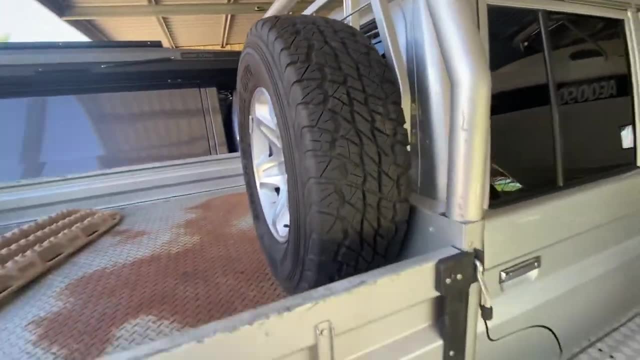 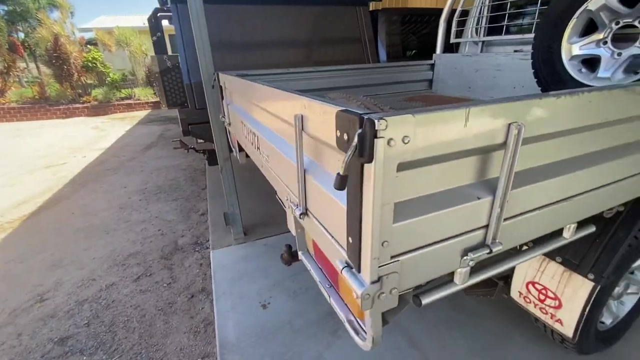 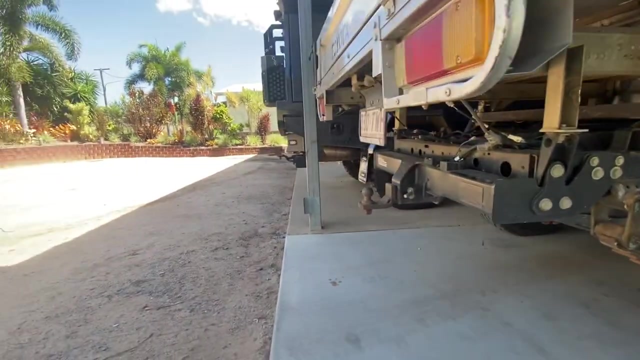 For that there's probably- I don't know- 100 mil in that to the roof section. That's the bigger cab ram to a 79. A standard Toyota tray. And have a look at the difference here. Look where the table is. his table's tow bar's, right under mine, sticks out loud with the tray. 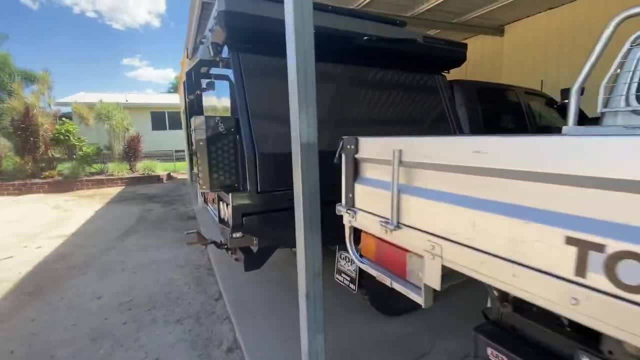 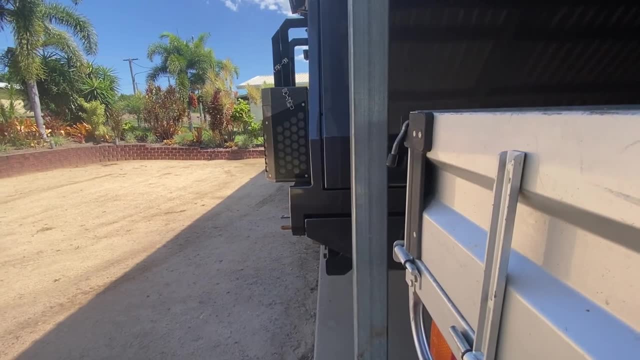 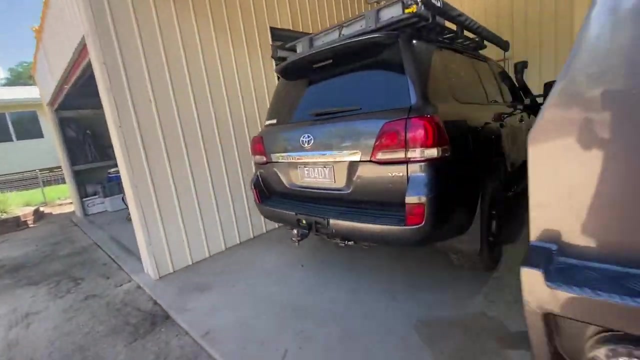 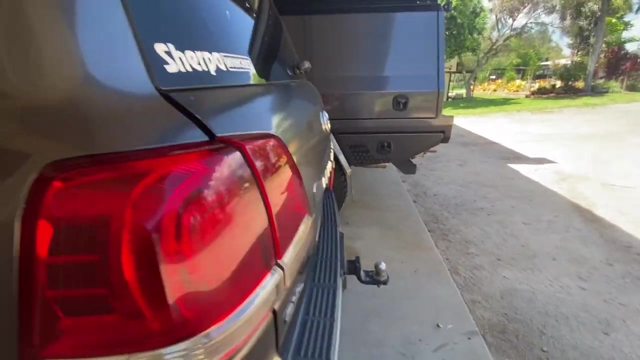 Stock standard short body: Toyota body. If you look there there's probably I could measure it. I'm gonna say 200 mil there difference Between the back of that canopy, the back of that, And the difference is there. the 200 comes in level with the wheelbase. 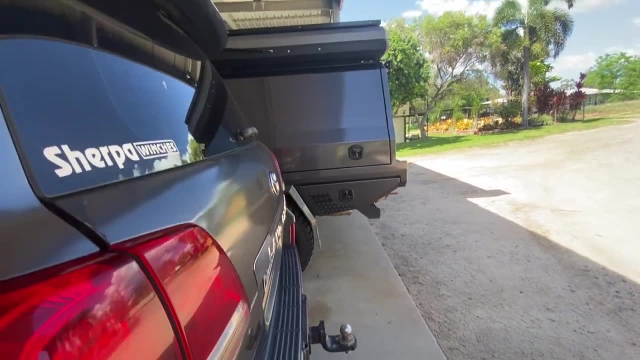 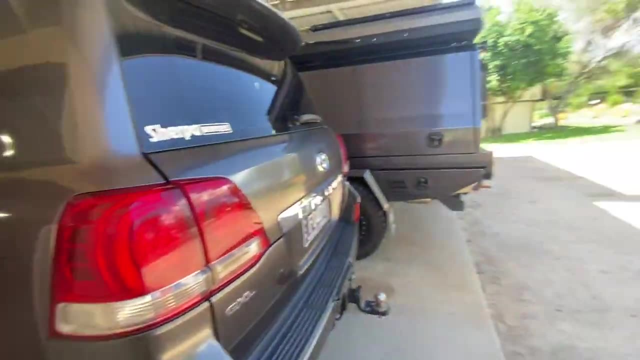 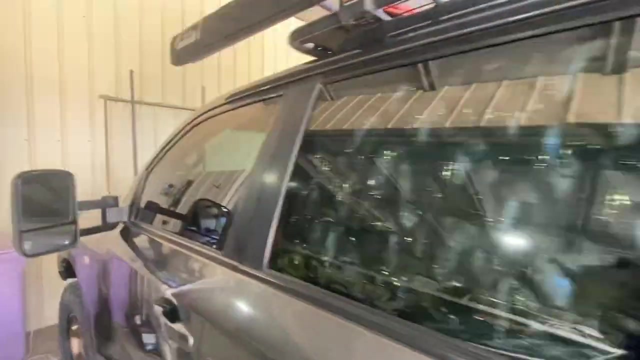 The rear of the car comes in level with the wheelbase of the ram. That's the difference in the size. So once you get a Land Cruiser extended, they are exactly the same length As the ram. Now I just showed you the cabin size. 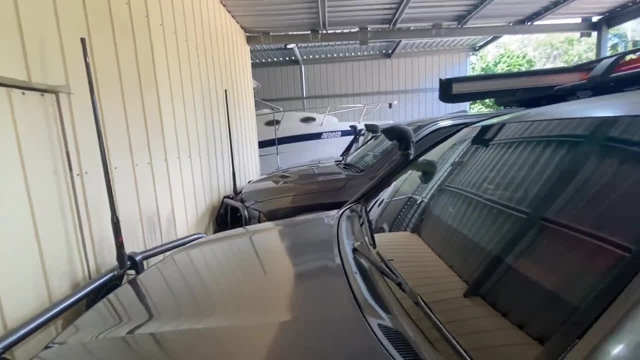 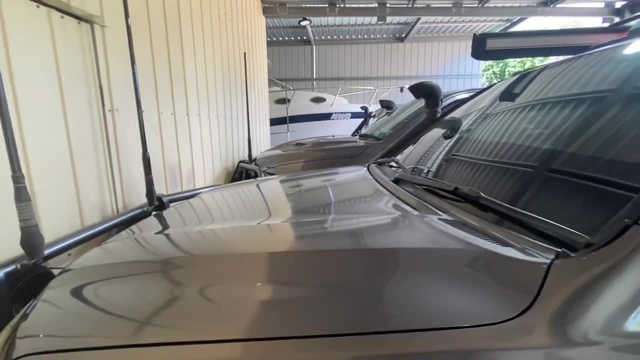 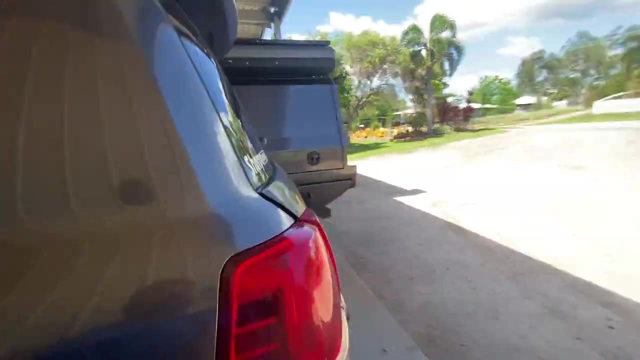 And physical distance. The actual look 79's actually a steeper windscreen Than the two cars parked side by side. I just wanted to show you a comparison. And people say the ram's too big, it's too long. Shows here in the real world. 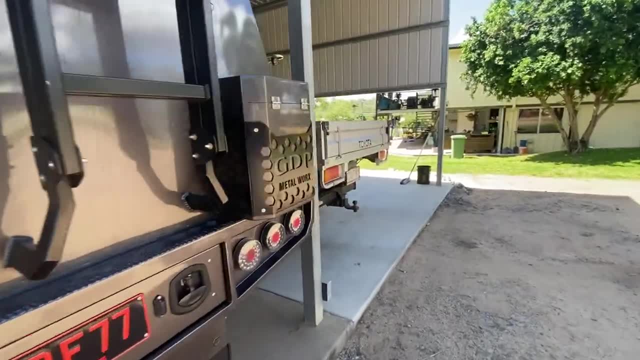 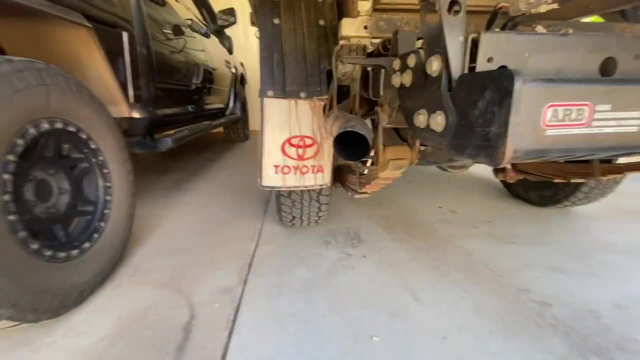 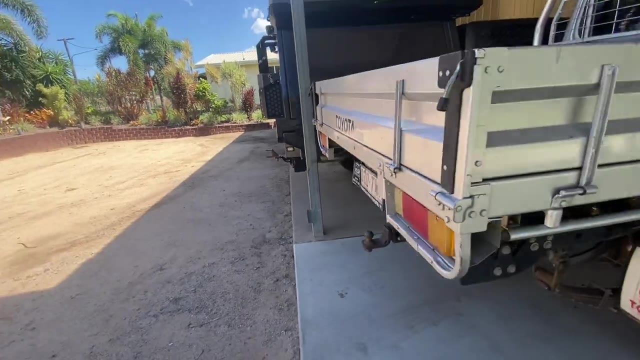 Against a 79, twin cab. The length is not That much different And the wheelbase is out behind it, Not tucked right up underneath it, And the tow ball is out There, Yeah, so The car Just done another trip. 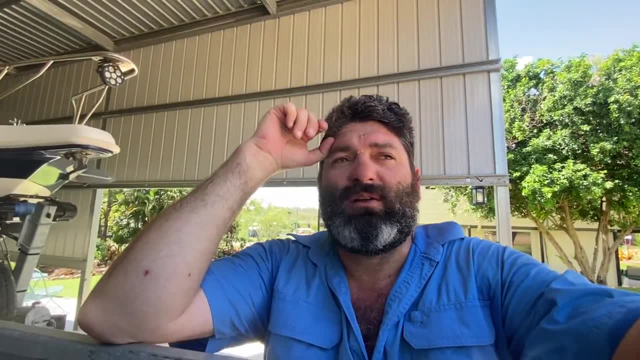 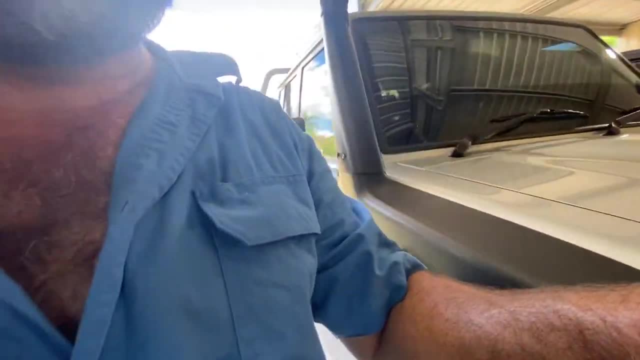 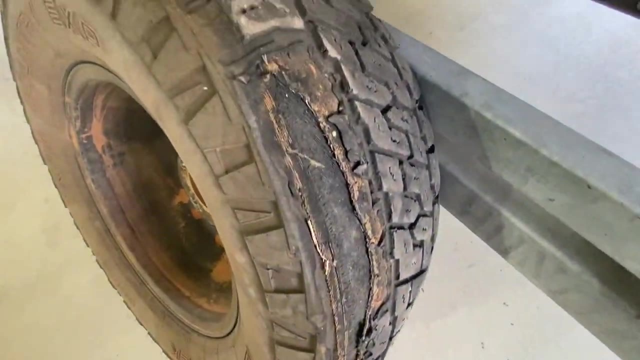 If you see on my YouTube channel, it's another trip up to the territory. We had a lot of harsh conditions this time, A lot of hard rock, Gravel rock. I'll just show you. Yeah, Dick's seat back. She went to shit. 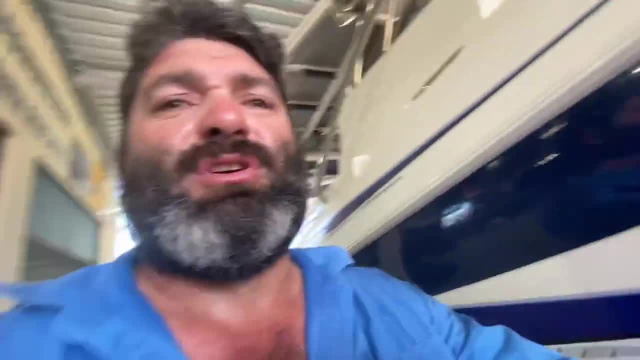 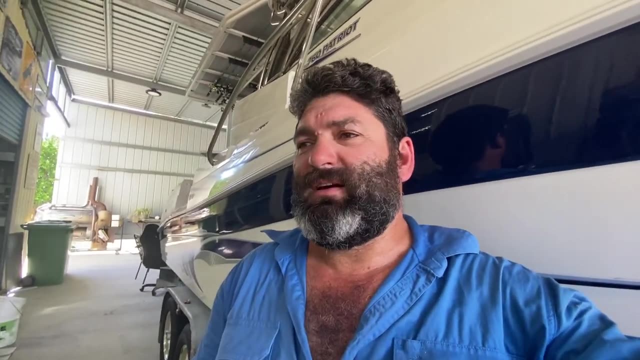 Destroyed that tyre And the other rear tyre has some chunks in it as well. The car went flawlessly. The air conditioner performed well, It was 43 degrees. The car rides excellent corrugation And just can't fault it. 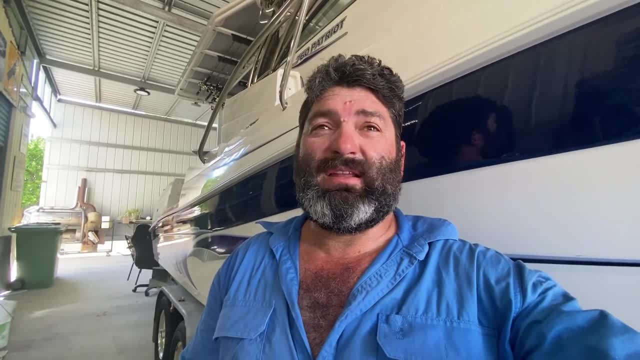 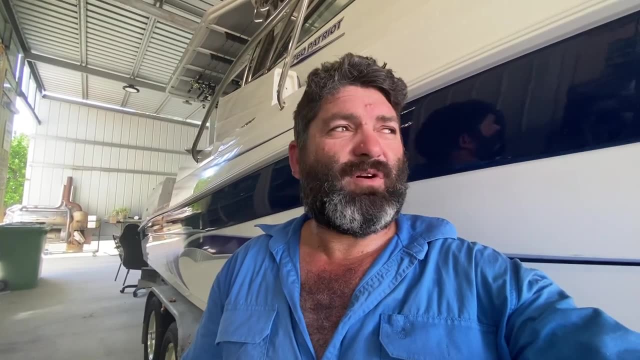 Excellent fuel economy, Getting around the 19 litres Towing the boat fully loaded, Through gullies and In the hot conditions. So 19 litres to the 100.. Done about 5,000 kilometres And yeah, still can't fault it. 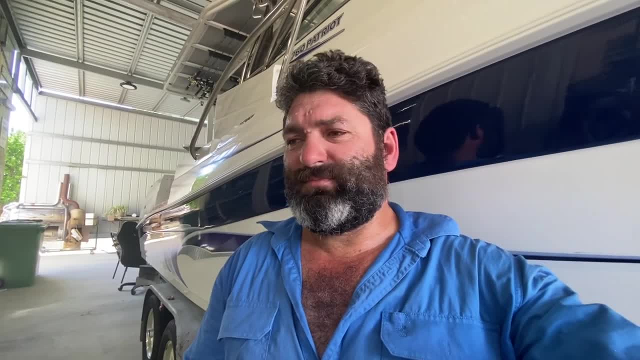 The car has been excellent in Australia. Got 53,000 Ks on it now And, yeah, absolutely just hasn't missed a beat, Hasn't let me down And the roads where we're going on is horrendous corrugation. 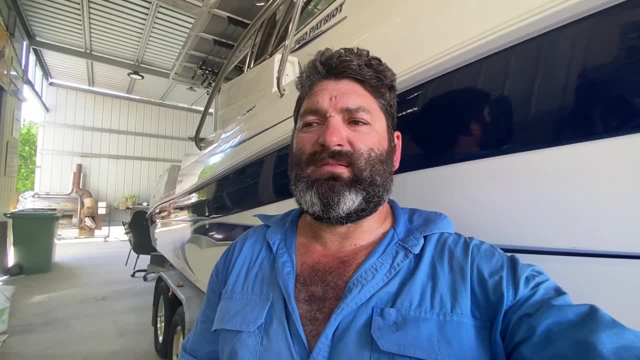 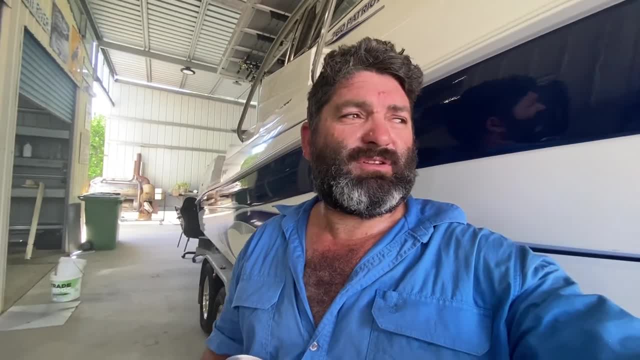 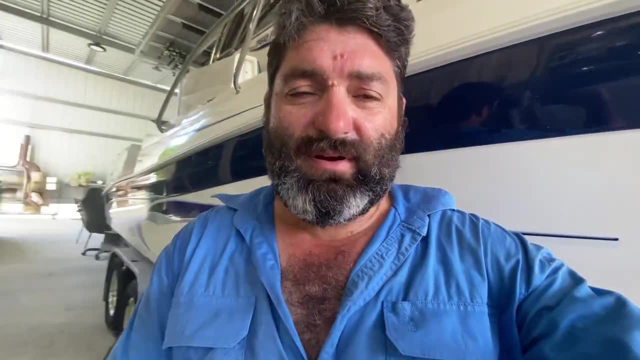 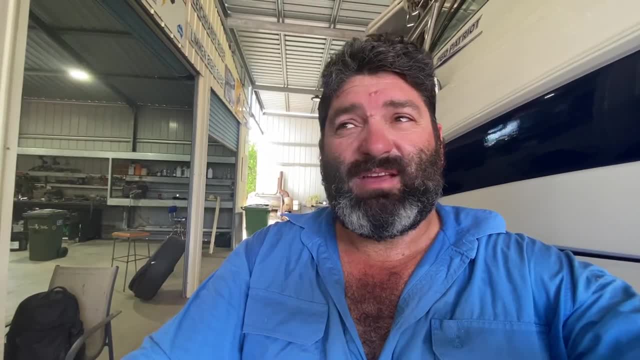 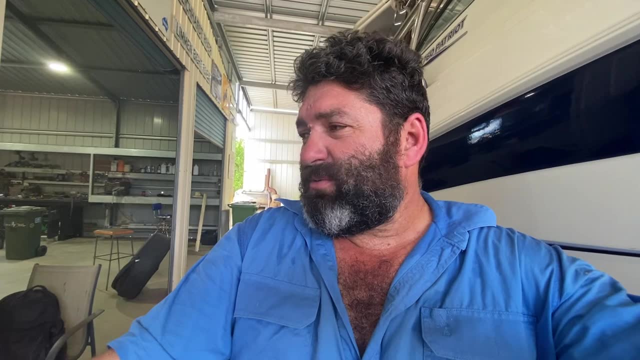 53,000 Ks Probably done. Had to be 30,000 Ks of that, Or at least 20,000 Ks of that. More hard dirt work, Yeah, trucking and bush work and pickup and everything and it's been great. 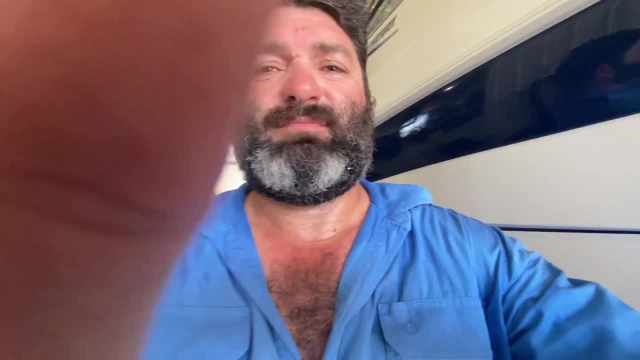 So cannot fault it Hiring out. 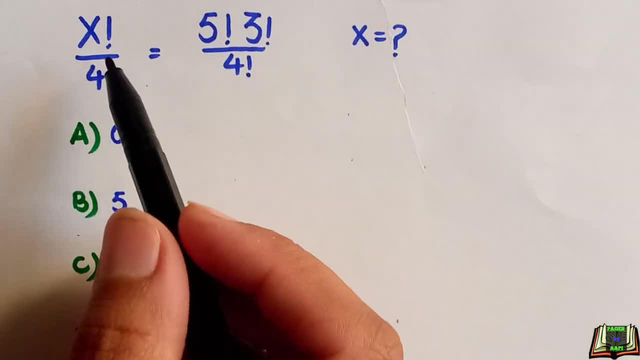 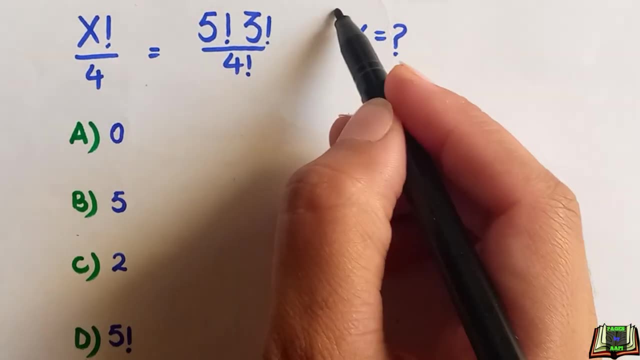 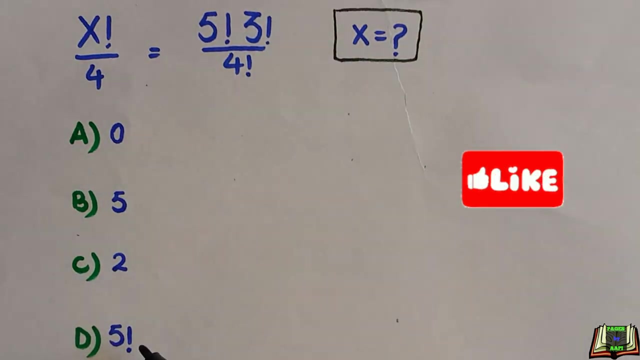 Welcome you to another interesting factorial question. If x factorial over 4 is equal to 5 factorial times 3 factorial over 4 factorial, then we have to find x. in this question Four values are given and we have to find the correct one. So let's see solution. It is given that x factorial